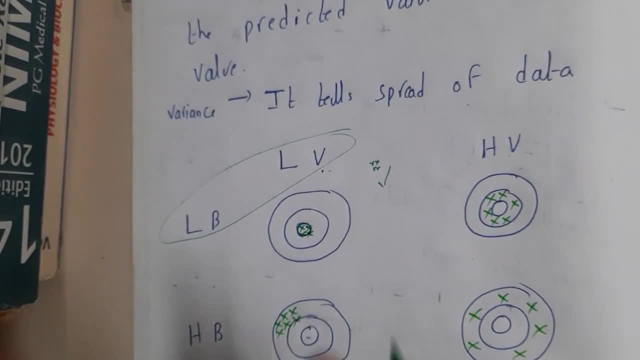 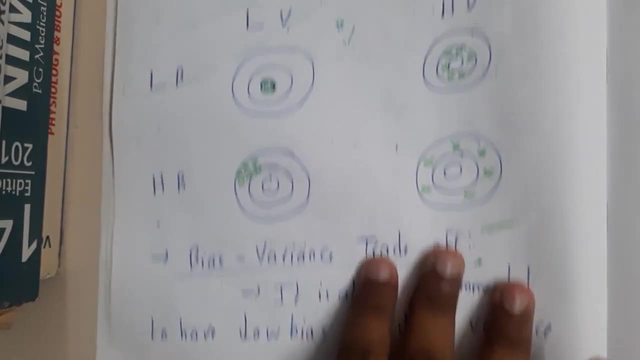 low variance and low bias. guys Got it? Yes. So that is what I was trying to say: okay, Yes. So if you check the next topic, that is nothing but bias variance trade-off. So this thing says about this: only guys, okay, Got it? Yes, So it is also recommended to have a low variance. 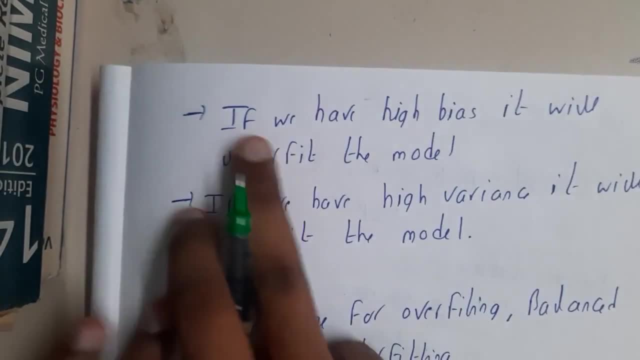 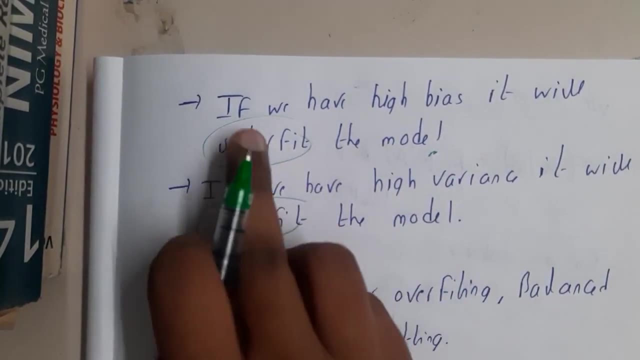 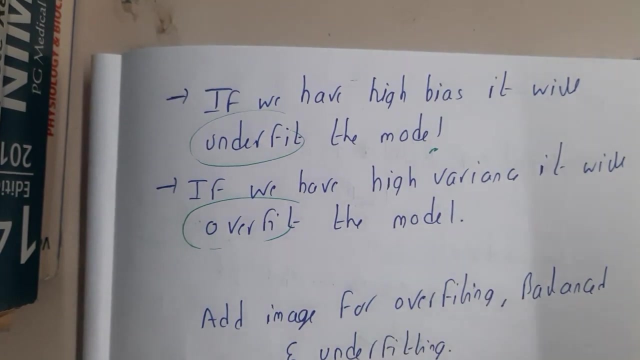 okay. So if we have high bias, it will underfit the model. okay, Guys, I will be showing you an image just for underfitting and overfitting, don't worry. So if we have high bias, we are going to underfit the model And if we are having high variance, we are going to overfit. 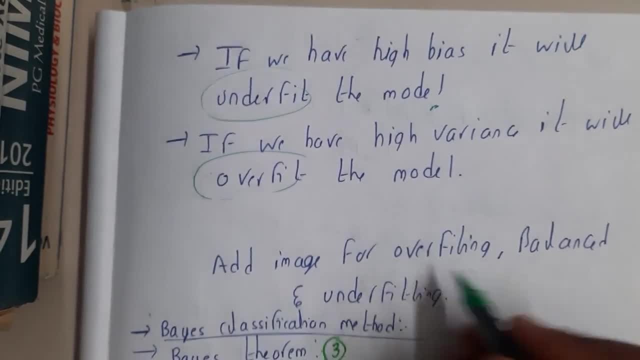 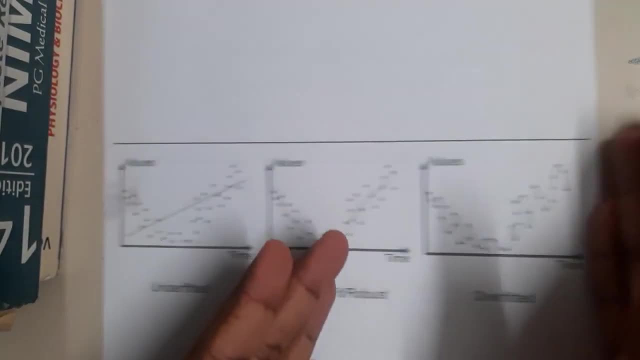 the bias. okay, So basically, you will be having a doubt that what is this overfitting, what is this balanced and what is this underfitting, right, Yes? So what is a balanced? so let us start from overfitting, guys. So overfitting is a state in which your graph or your line will try. 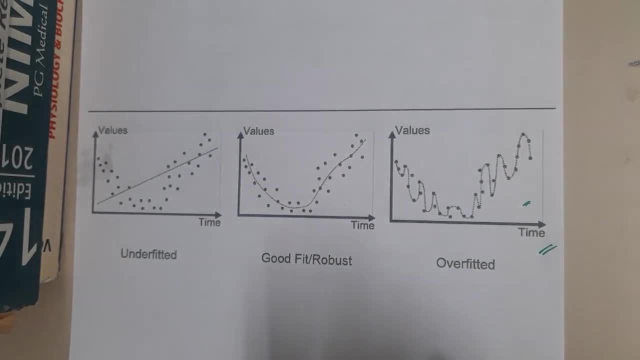 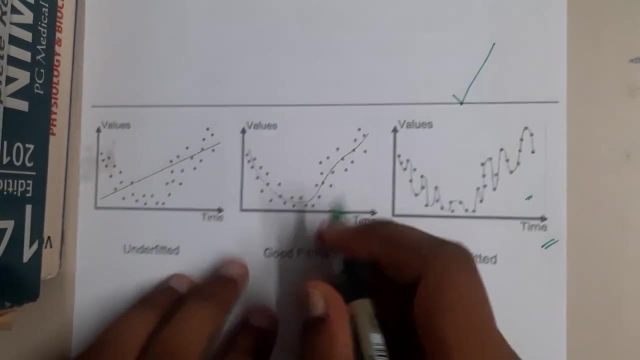 to connect each and every point. So if you notice here it is trying to connect each and every dot, right? Yes, So this concept is called as overfitting guys, okay. Similarly, if your graph is in a proper structural way and it is touching some points, it is not touching all the points. 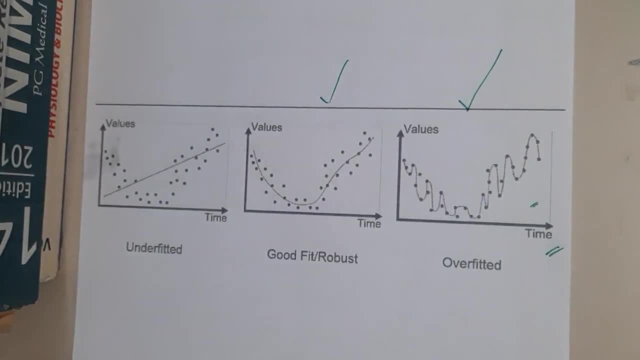 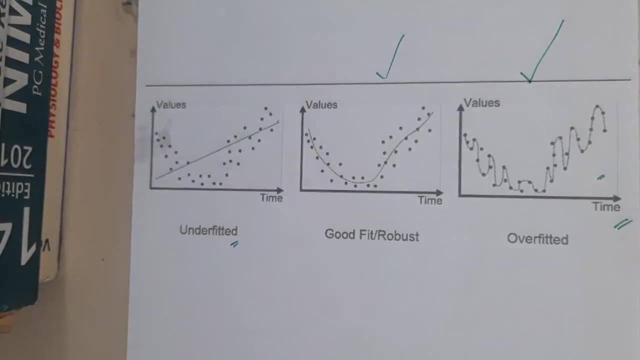 or it is not missing all the points. that is a good or robust graph, guys. When your graph is not touching any point, like see here, the point started from here to here and the line is going from here. So that is not a good thing, right? Yes, So that is nothing but the underfitted graph. 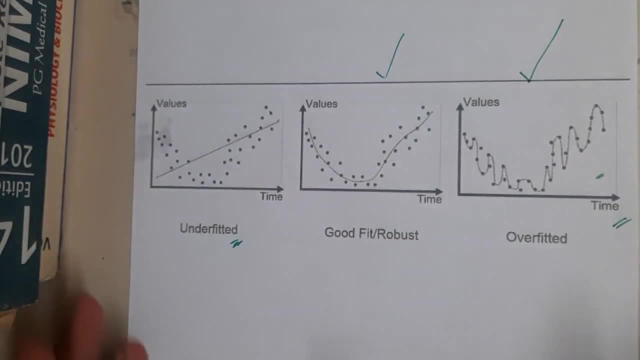 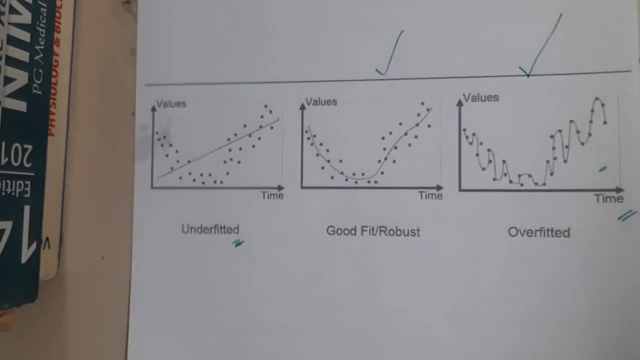 okay, I do not know exactly how you can write the definitions for them, guys, but with the diagrams it is really easy to explain. So that is the reason why: draw the diagram and explain in your own words, guys. okay, Yes, So I hope everyone got a clear idea about these three graphs. 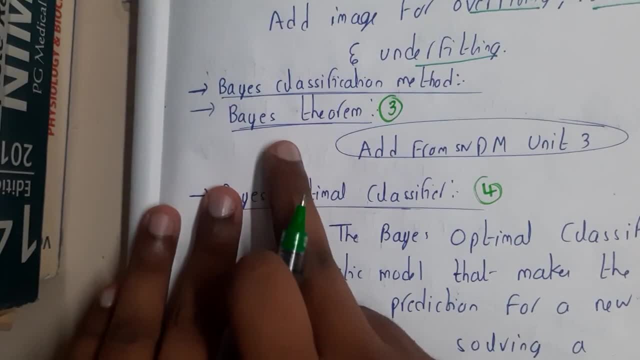 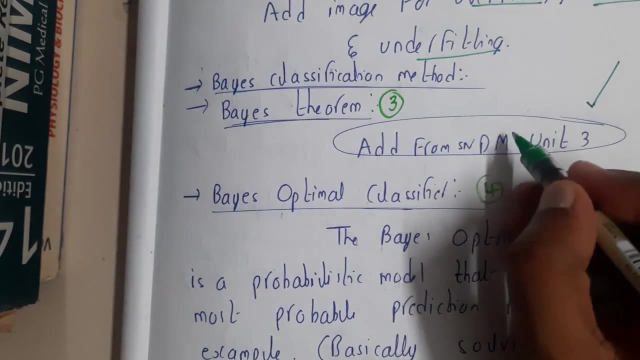 So in the next lecture we will be continuing with the Bayer's classification and inside Bayer's classification we will be discussing about Bayer's theorem Guys. mostly I will be connecting you back to a video which we have already done in the data mining guys. okay, 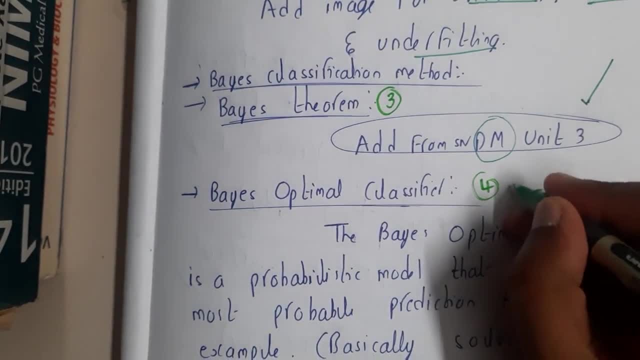 As I do not want to repeat the videos again and again. okay, In the next lecture we will be discussing about Bayer's optimal classifier. okay, Yes, So let us meet in the next lecture, Thank you. Thanks for watching.